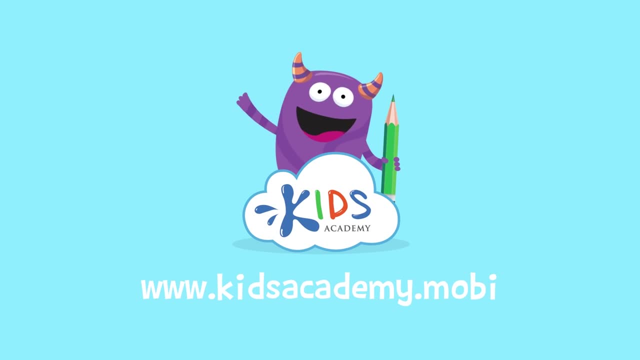 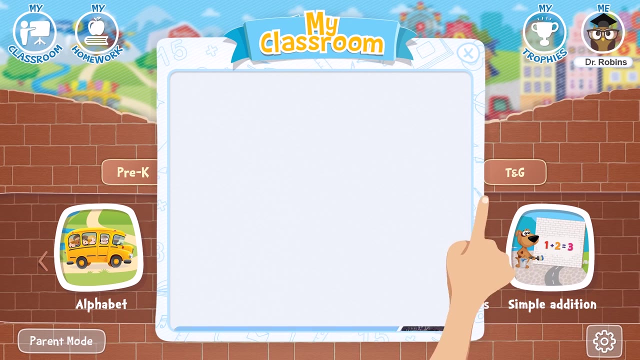 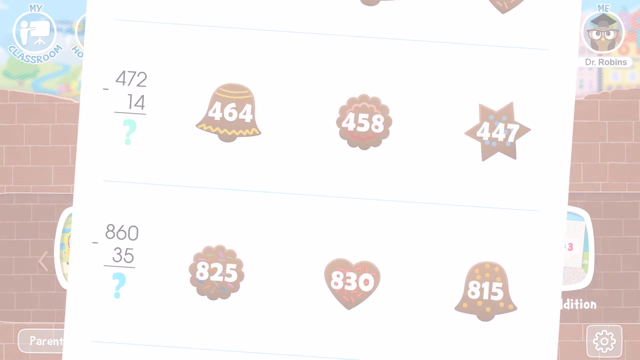 Welcome to kidsacademymobi. Hello everyone, Let's open the worksheet. Don't forget to like this video and subscribe to our channel. You can find the link to this app in the comments below. Today, we're going to be looking at a worksheet. 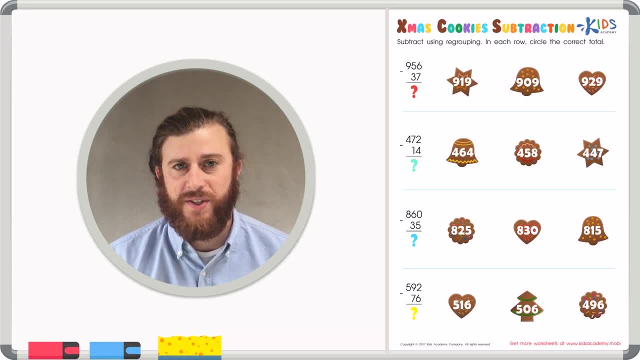 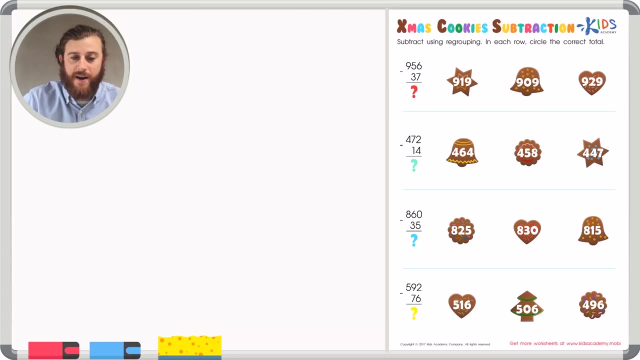 called Christmas Cookie Subtraction. Let's read the directions and look at an example so that way we're ready to solve the problems on this worksheet. Subtract using regrouping and each row circle the correct total. Let's look at an example before we get started. Let's take, for example, that number: 321 minus. 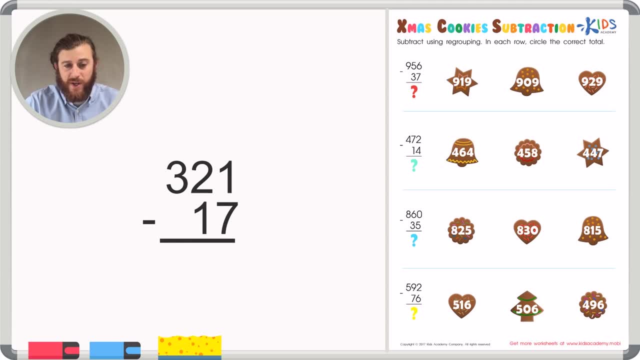 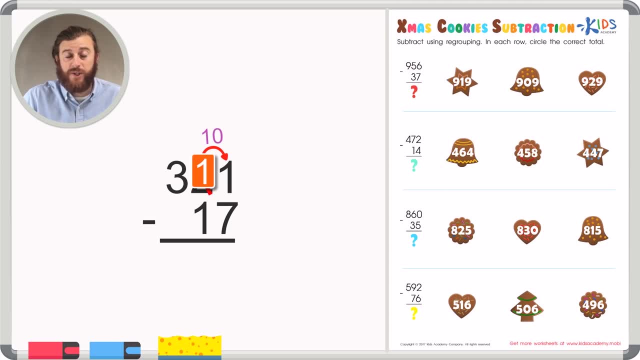 we're going to have to give to the 1 in the ones place. 10 plus 1 is 11, so the 1 just becomes 11.. Now you can take away 7 from 11, because 11 has 7 to give. So let's count upwards from 7 to 11. 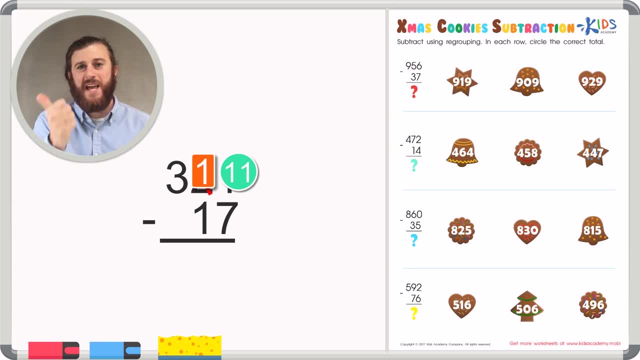 to see the difference between those two numbers: 7,, 8,, 9,, 10, 11.. 11 minus 7 is 4.. Now we can just move along and continue. subtracting: 1 minus 1 is 0, and 3 minus. 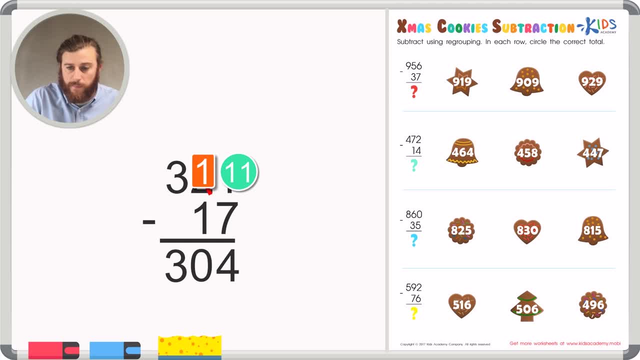 nothing is 3,, giving us an answer of 304.. Let's use this strategy of regrouping to help us solve the rest of the problems. Our first problem has us subtracting 956 minus 37. We have the same situation as we had in the example. The top number in the ones place is smaller than. 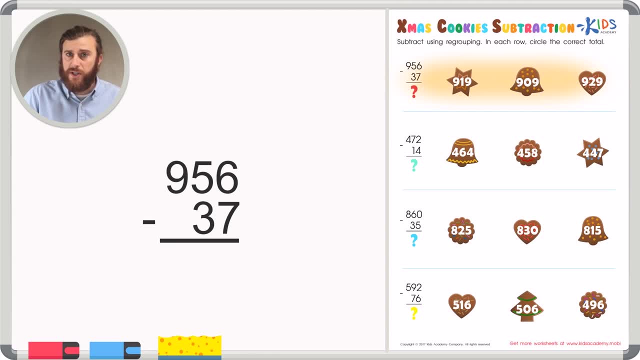 the number in the ones place. The top number in the ones place is smaller than the number in the, the bottom number in the ones place. So we're going to look next door to the tens place and borrow a ten from five. Fifty or five will become four and that ten that we borrowed 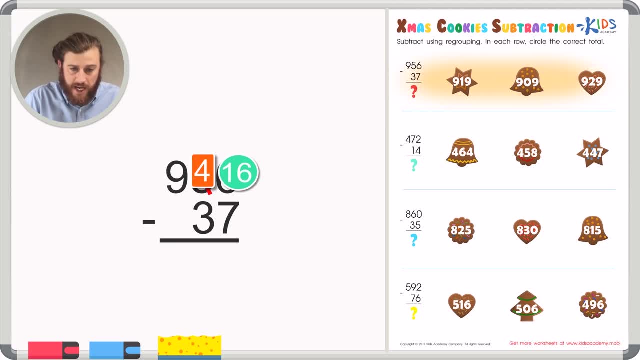 will add to six, and six plus ten is sixteen, So our six becomes sixteen. Sixteen minus seven is a problem in which we'll probably have to use our fingers, so let's count up from seven to sixteen. Seven, eight, nine, ten, eleven, twelve, thirteen, fourteen, fifteen. 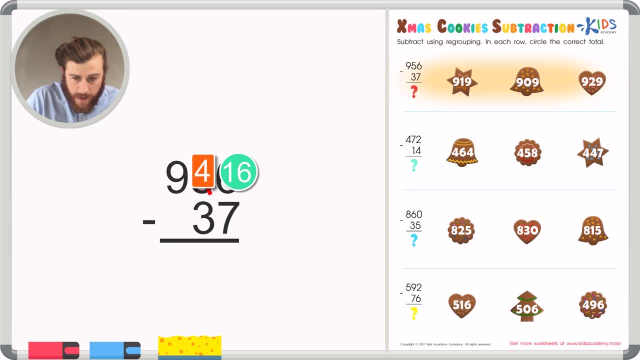 sixteen. Sixteen minus seven is nine, Just like before, we continue subtracting from right to left. Four minus three in the tens place leaves us with one and nine minus nothing in the hundreds place is nine, giving us a difference of five hundred and fifty-six minus. 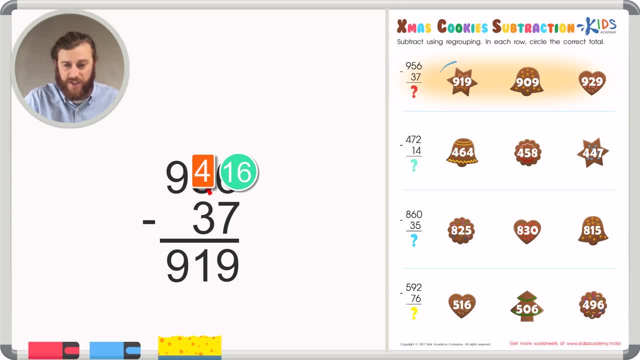 thirty-seven of nine hundred and nineteen. Our point is to be careful not to forget that the tens place is the ones place and that's our first answer choice. Let's go ahead and circle that. Our second problem has us subtracting four hundred and seventy-two and fourteen, A similar situation. The top one is smaller. 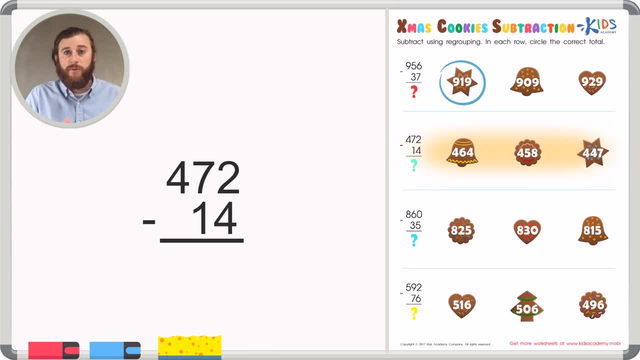 than the bottom one. You cannot take away four from two. Two only has two to give, so it must borrow from the tens place. If we cross out seven in the tens place, turn the seven into a six or seventy into sixty. 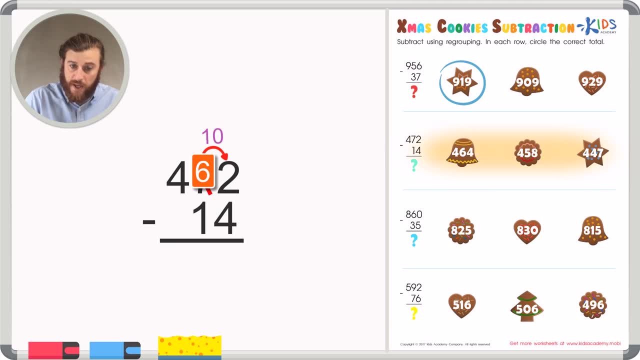 The ten that we borrowed we will give to the two, and that makes it a twelve, because ten plus two is twelve, Twelve minus four. again, we'll use our fingers Four, five, six, seven, eight, nine, ten, eleven, twelve. That gives us a difference of eight in the 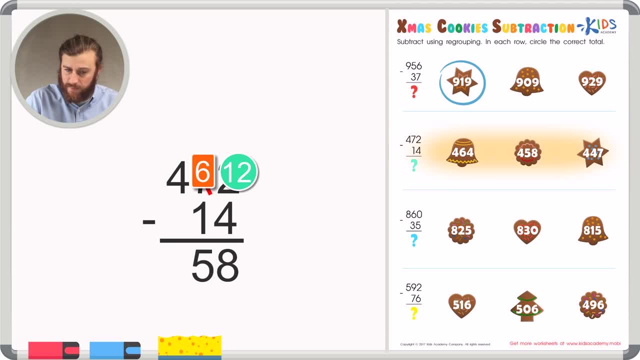 ones place. Six minus one is five. That's an easy subtraction problem. And four minus nothing is four, giving us a total or a difference, of four hundred and twenty-six. That's our answer. Eight hundred and seventy-eight, the second answer choice. Our third example has us subtracting. 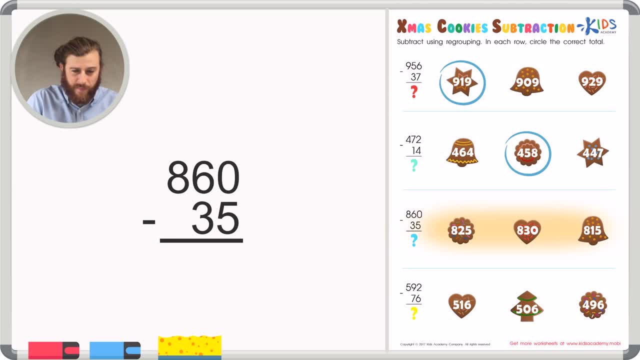 eight hundred and sixty minus thirty-five. I noticed that in the ones place there's a zero. It has nothing to give. so we're going to have to borrow from the tens place. We could borrow one ten from sixty and turn our sixty into fifty or five and give that. 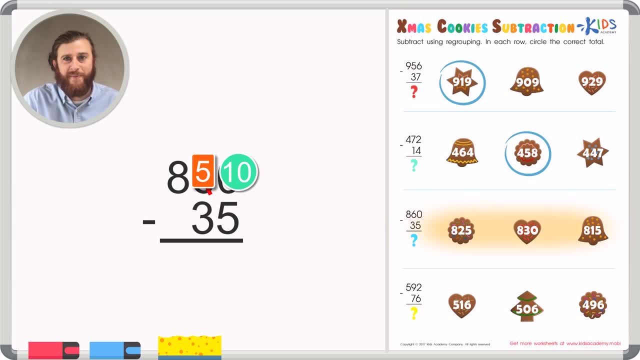 ten to the ones place Now we have ten minus thirty. eram gochisosama is 5.. That's an easy subtraction problem. 10 minus 5 is just 5.. Subtracting from right to left, 5 minus 3 is 2. And 8 minus nothing is 8, giving us a difference of 825, our first 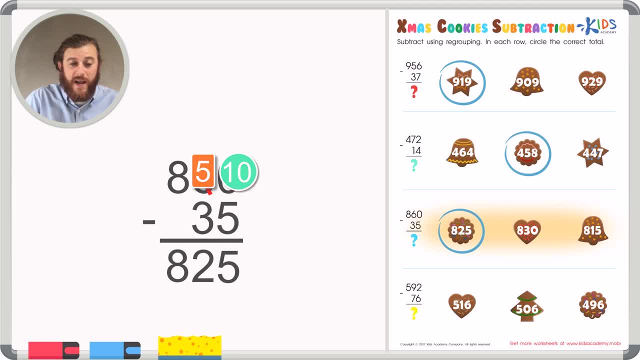 answer choice. And finally we have 592 minus 76.. In this problem, again, the top ones place number is smaller than the bottom ones place number. We're going to have to borrow from the tens place, but he doesn't mind, He's got plenty to give. Let's take away one 10. 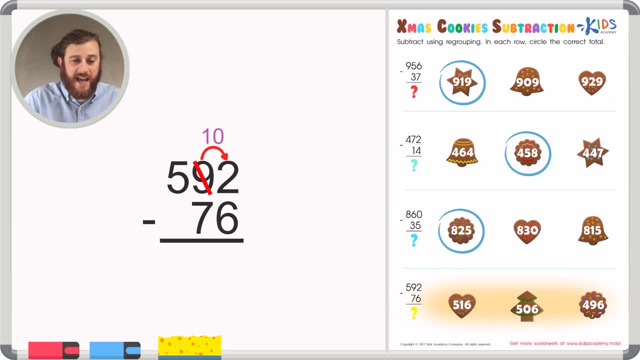 from 9,, which is really representing 90, and turn it into 8,, which now will represent 80. We'll take that 10 and give it to the 2 in the ones place, making 2 a 12.. 12 minus 6. 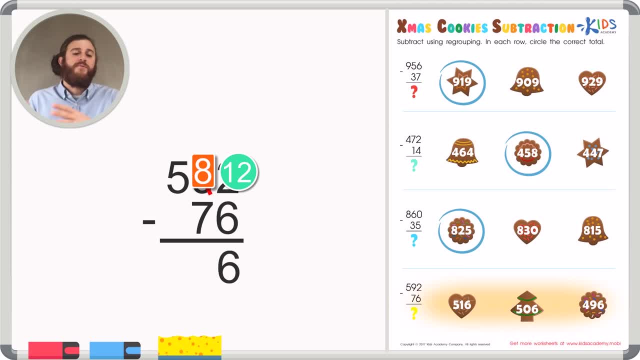 is 6.. We can continue subtracting from right to left. 8 minus 6 is 6.. We can continue subtracting from right to left. 8 minus 6 is 6.. We can continue subtracting from right to left. 8 minus 6 is 6.. We can continue subtracting from. 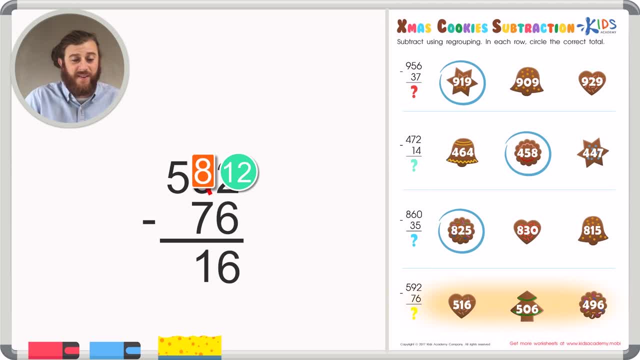 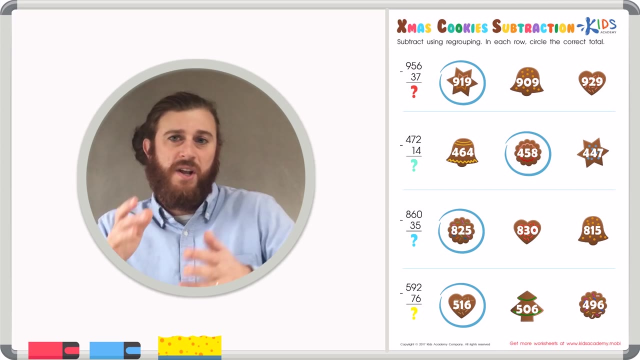 right to left. 8 minus 7 is a difference of just 1.. And 5 minus nothing is just 5, leaving us with a total difference of 516,. our first answer choice. Remember, boys and girls, if the top number is smaller than the bottom number, even if it's in the ones place. 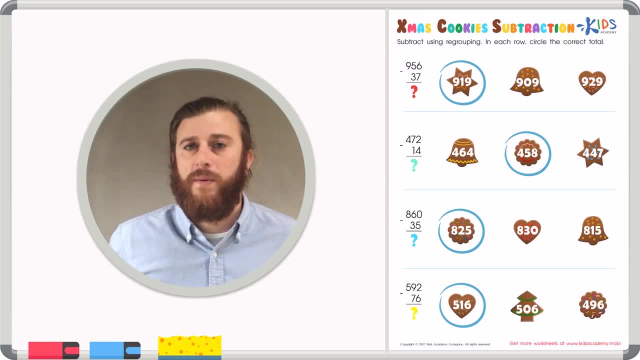 the tens place. you have to borrow from the place next door. You're borrowing the value of that digit. So if you borrow 1 from the tens place, you're really borrowing 10.. So you can add 10 to the previous place. Thanks for watching, boys and girls. We'll see you next time. 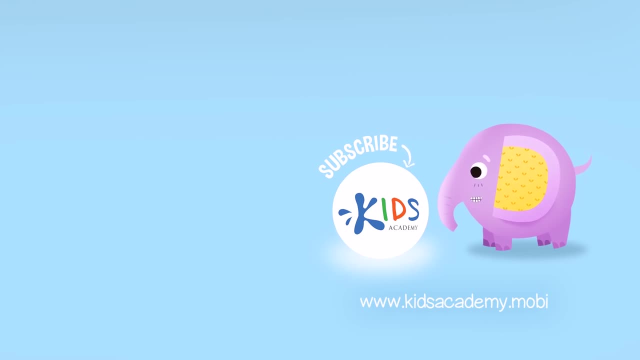 Like us and subscribe to our channel. Find links to our apps and comments below.